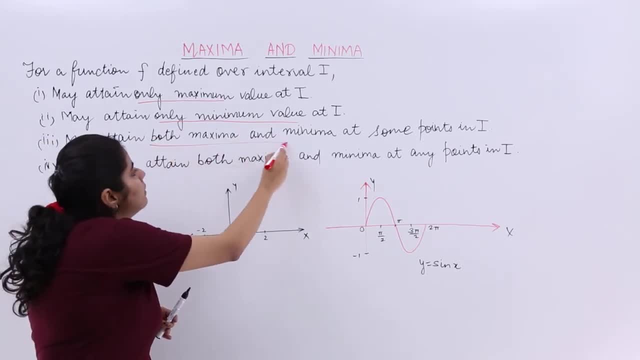 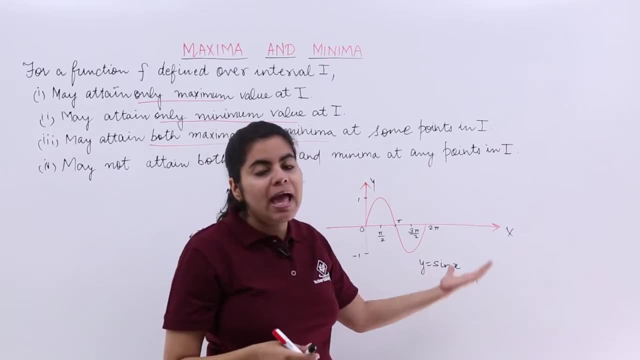 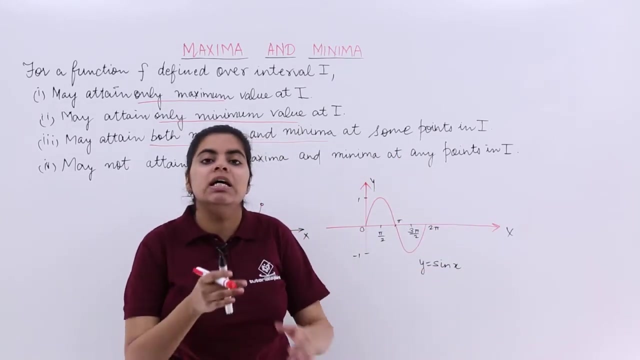 attain both maxima and minima. So both maxima and minima. some examples would be trigonometric functions. Suppose I am taking the graph of y is equal to sine x. This is the graph. And now the sine x curve is something like this that you already know. It alternately goes up and down, up and down Right Now. 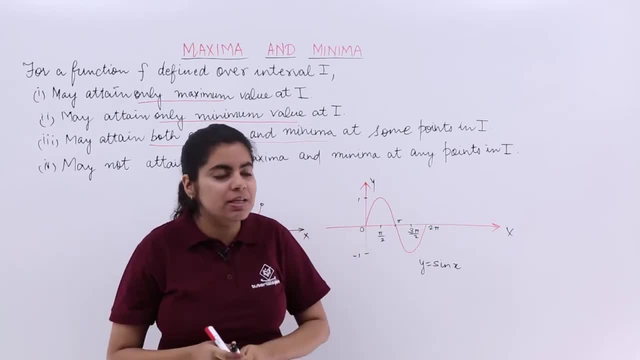 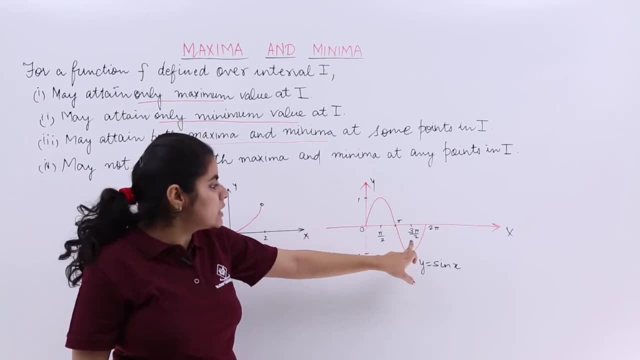 suppose I have to take only the interval 0 to 2 pi into consideration. so the graph would be like this: At 0 it is 0. only Sine pi by 2 is 1.. Sine pi is again 0.. Sine 3 pi by 2 is minus. 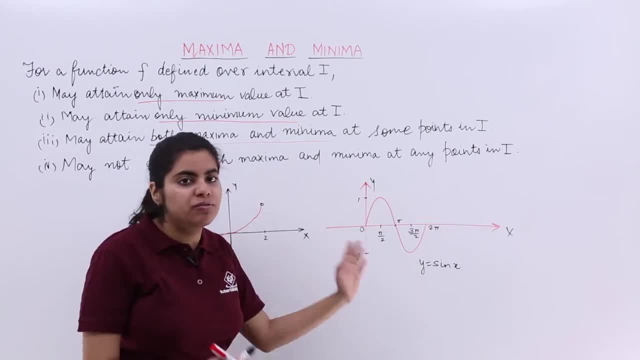 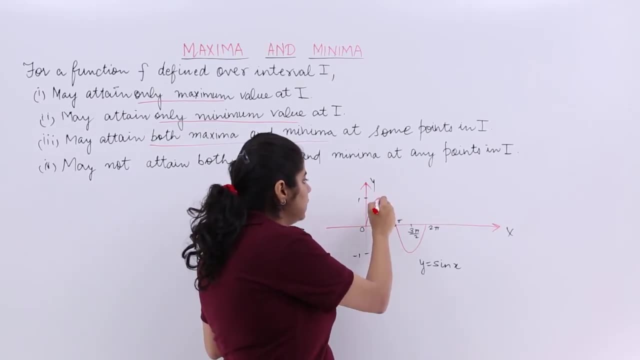 1 and sin 2pi is again 0.. A very roughly made graph only for understanding. Now you see that. what is sin pi by 2?? It is 1.. It is gaining the highest value. sin x is attaining the highest value. 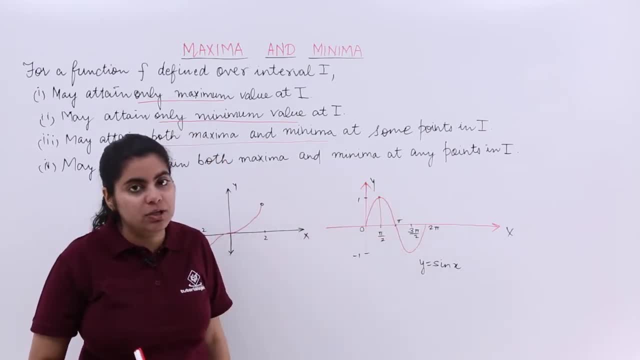 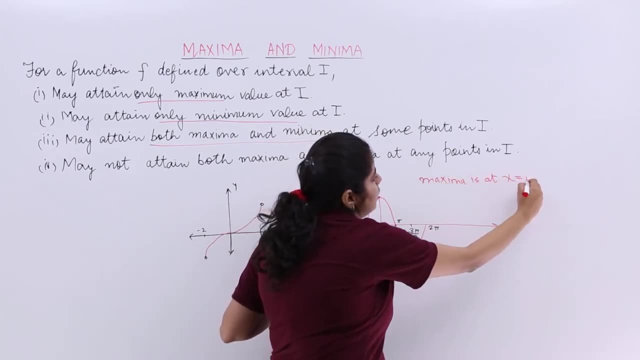 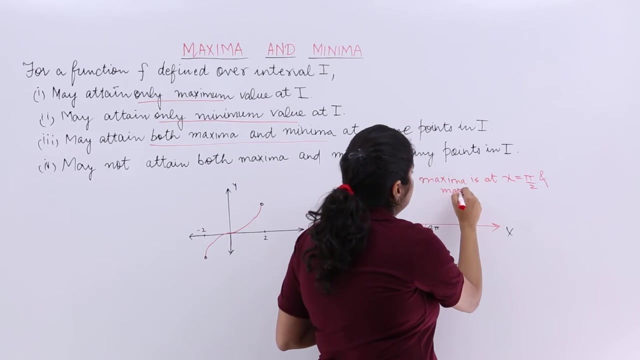 1 in the interval 0 to 2pi at pi by 2.. So I say that maxima is there and the maxima is at x is equal to pi by 2, and it is what? And it is 1 and maximum value is 1, right, We are talking. 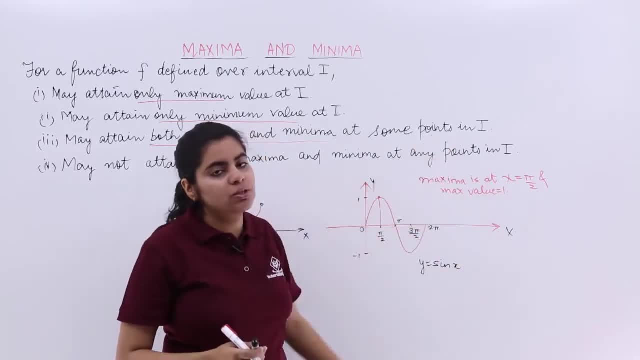 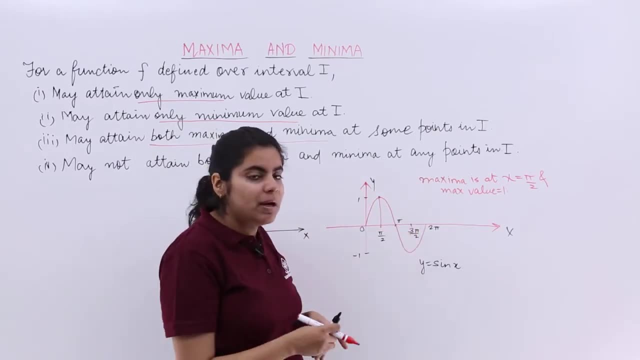 only about 0 to 2pi, mind it. Where i is the interval here? 0 to 2pi is the interval. Let's talk about now minima. Does minima also exist? Yes, when we move forward we see that at 3pi by 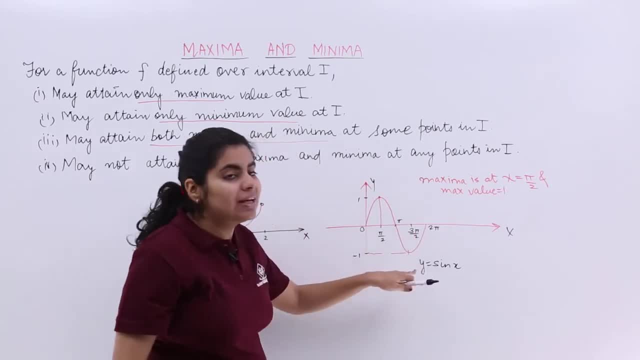 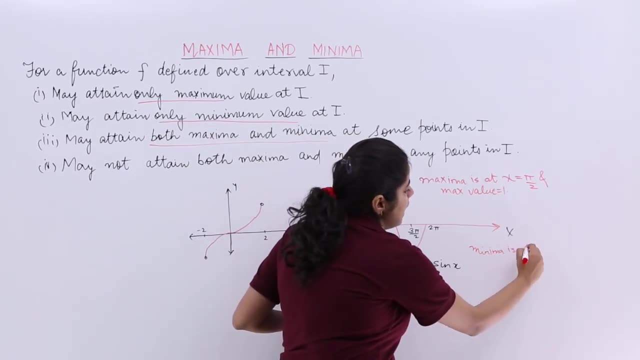 2, the value corresponds to minus 1 and minus 1 is the least value into consideration in 0 to 2pi. So I say that minima is at x is equal to minus 1. and what is the minimum value? Sorry, minima is. 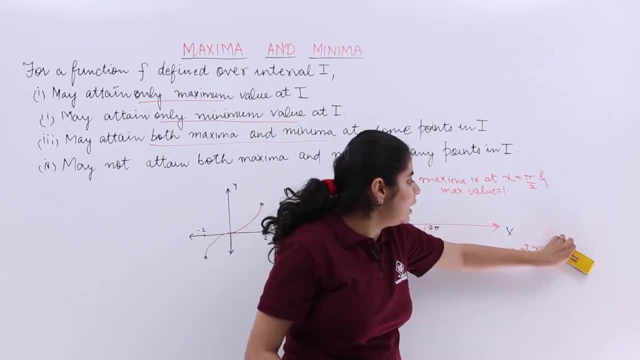 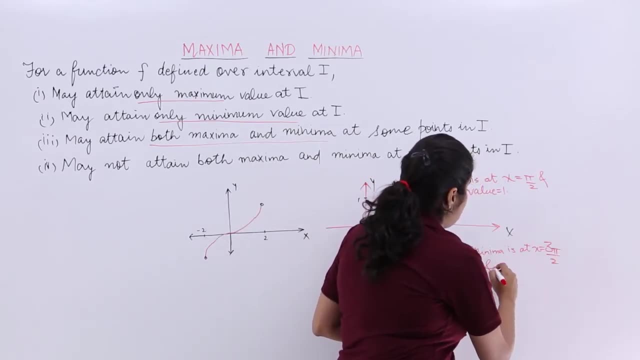 at x is equal to 3pi by 2. and what is the minimum value? It is nothing but minus 1.. So you see that both maxima and minima exist. So 3pi by 2 and it is equal to minus 1.. So sin x or similarly, cos x. 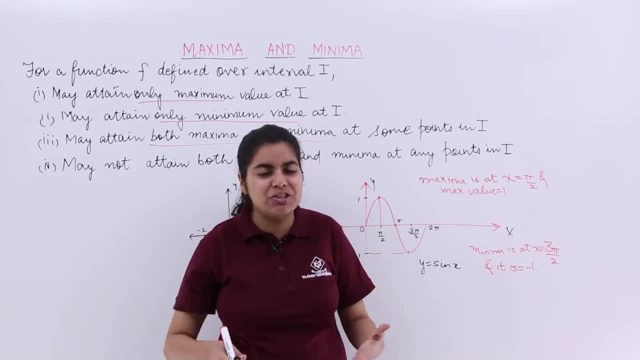 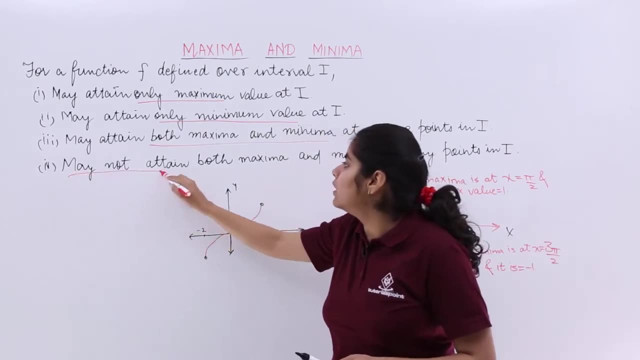 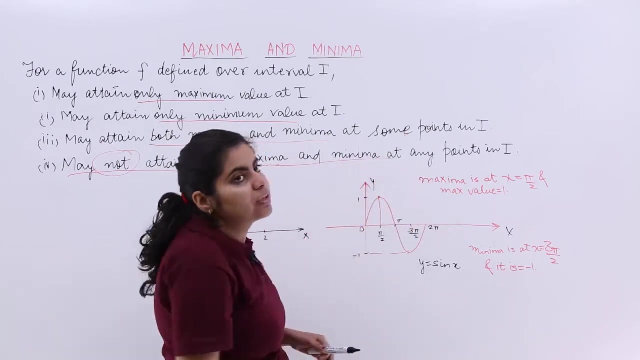 is such kind of a graph, One example of such kind of a graph, which has both maxima and minima. Next, sometimes it may also happen that the graph may not attain both maxima and minima, means it may not have maxima, it may not have minima. What kind of?